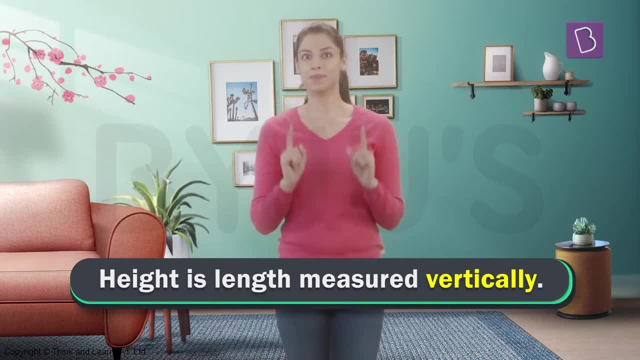 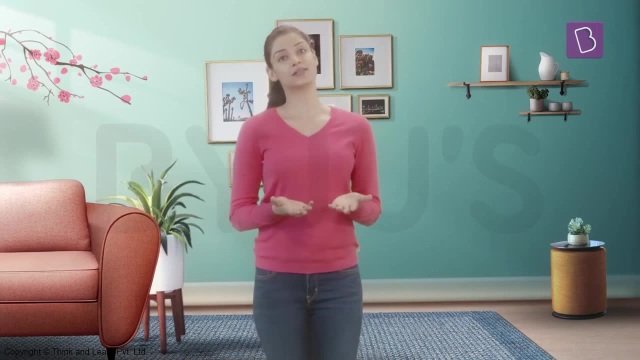 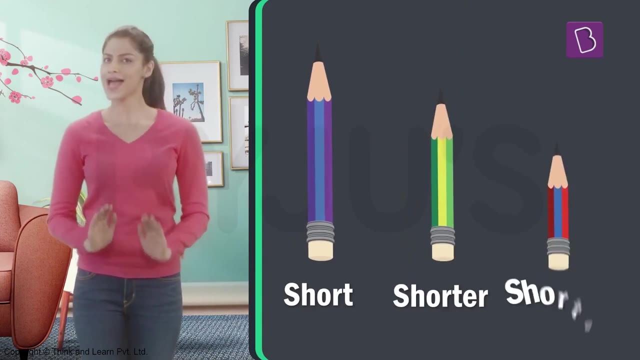 height of something is nothing but a number. So we can measure the height of something by measuring, but measuring its length vertically Simple. Now we use terms like tall, taller and tallest, or short, shorter and shortest, to compare heights of different objects. 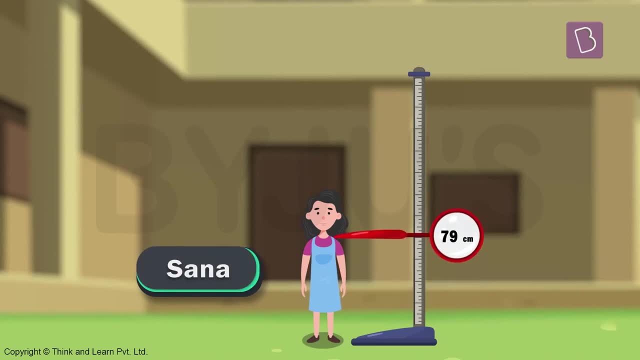 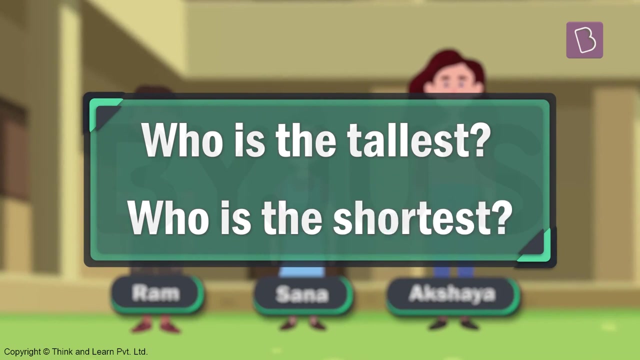 For example, Sana's height is 122 cm, Ram's height is 132 cm and Akshaya's height is 144 cm. Then, out of all these three, who is the tallest and who is the shortest? Clearly, Akshaya is the tallest. 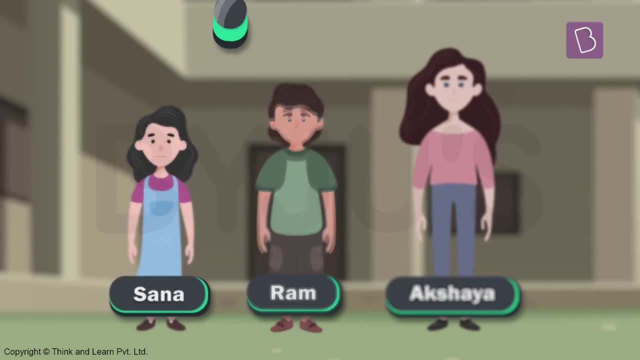 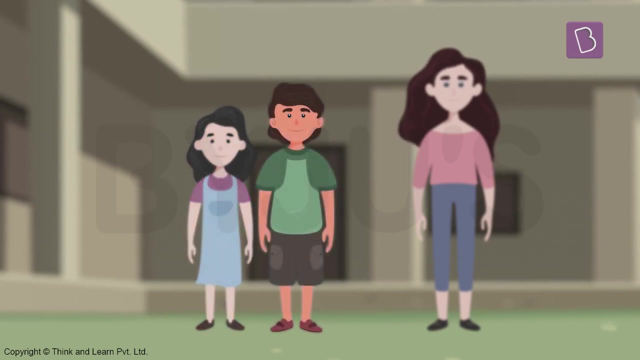 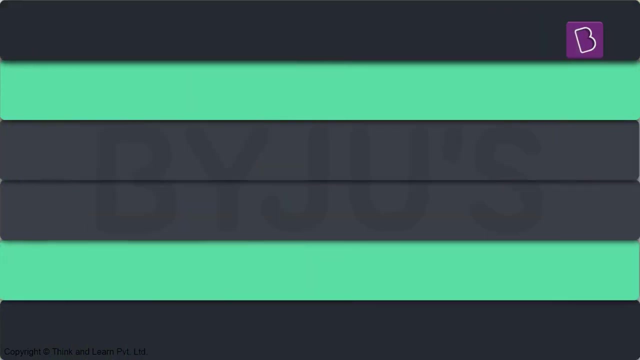 Ram is taller than Sana and Sana is the shortest. Therefore, while lining up for the morning assembly, Sana will stand in the front because she is the shortest, followed by Ram, and at the end will be standing Akshaya. Now, if I ask you, 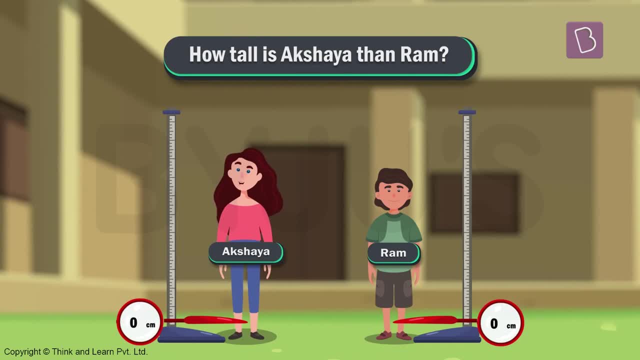 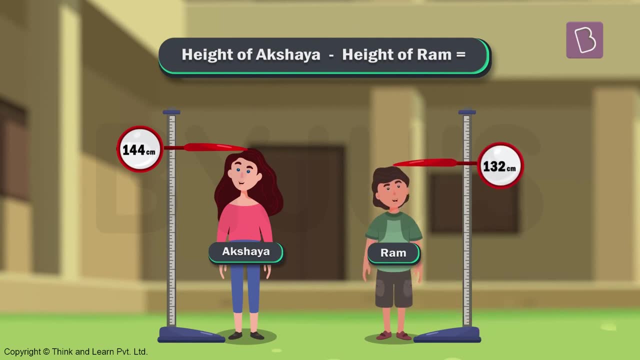 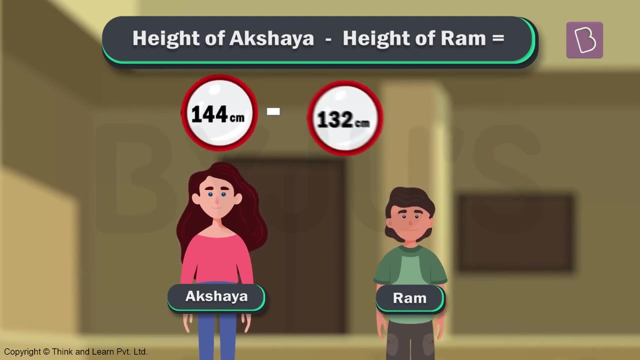 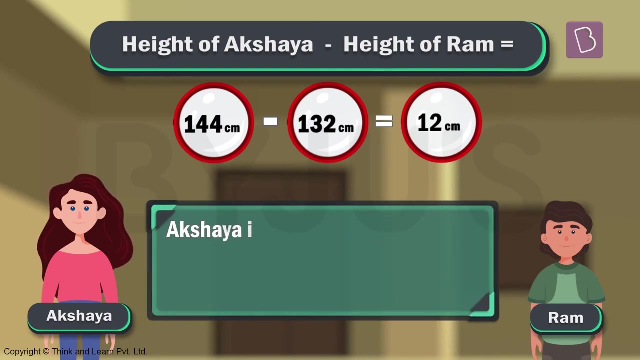 how tall is Akshaya than Ram? It will be the height of Akshaya minus the height of Ram, Which is 144 cm, minus 132 cm, which is equal to 12 cm. Therefore, Akshaya is 12 cm taller than Ram. 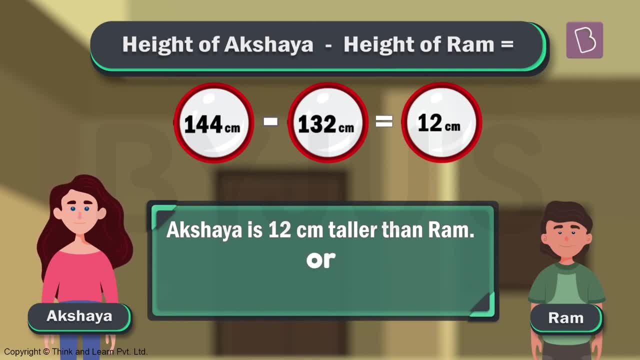 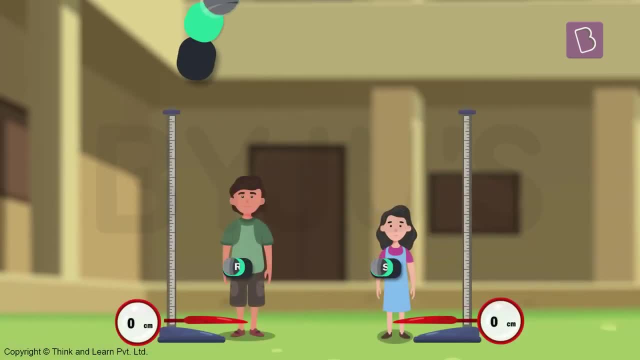 Or in other words, we can say that Ram is 12 cm shorter than Akshaya. Now how tall is Ram? Let's see How tall is Ram than Sana. It will be the height of Ram minus the height of Sana. 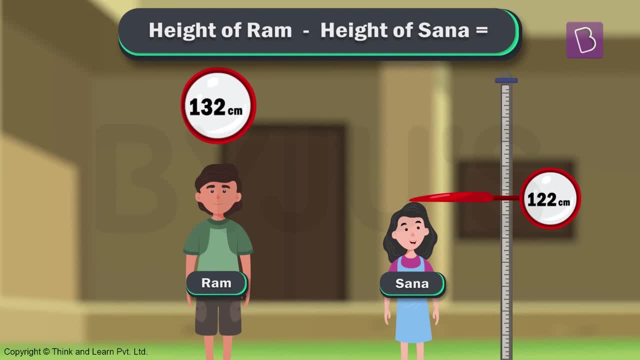 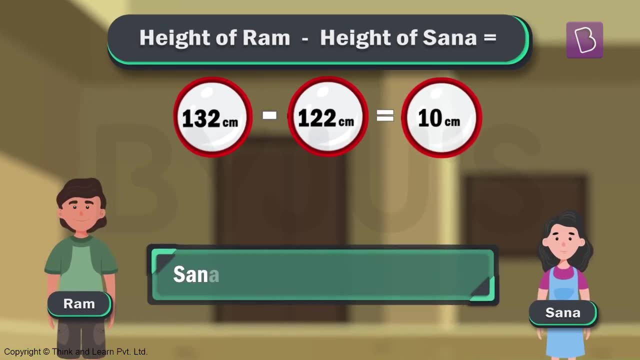 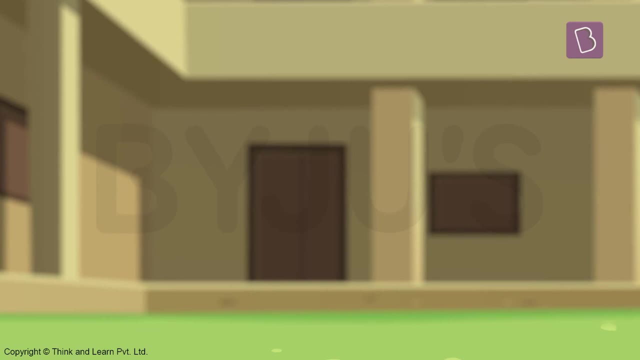 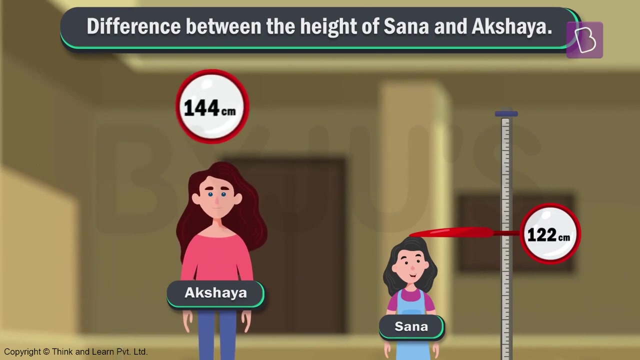 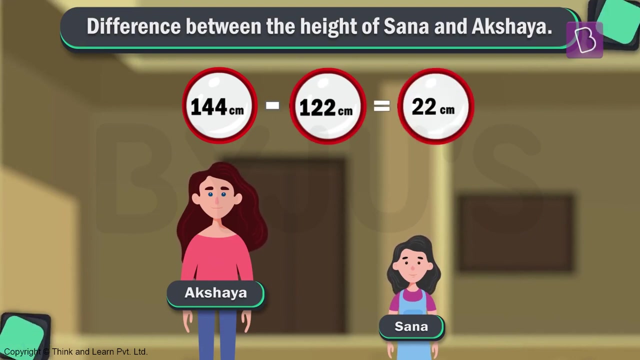 which is 132 cm minus 122 cm, equals to 10 cm. Therefore, Sana is 10 cm shorter than Ram. Similarly, we can find the difference between the heights of Sana and Akshaya, Which will be 144 cm minus 122 cm equals to 22 cm.